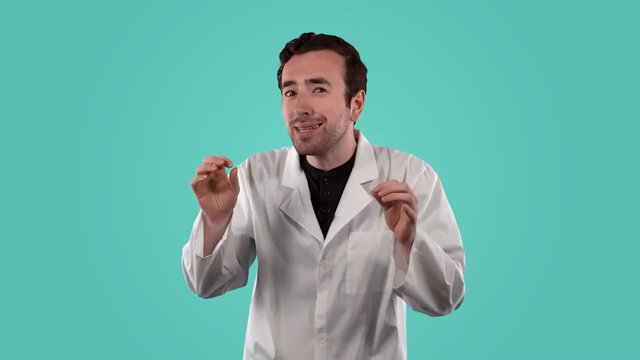 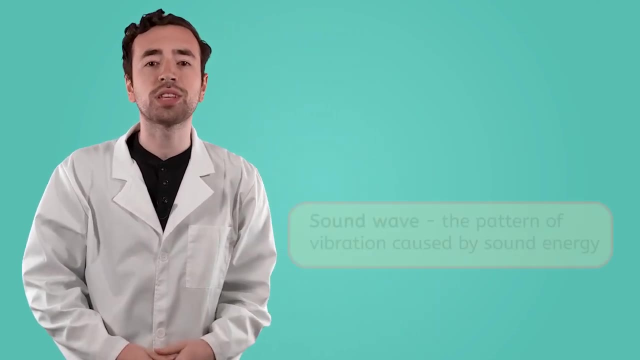 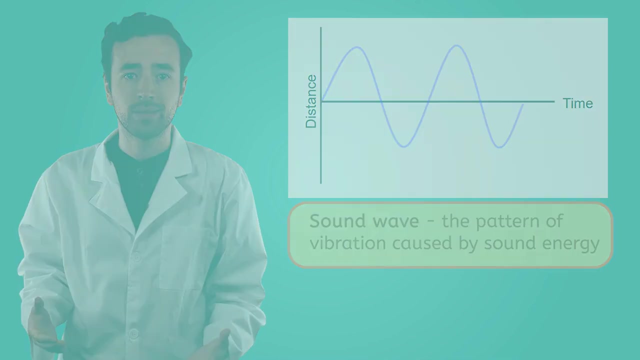 through a huge movement or just wiggling, By following how each particle of matter moves with sound vibrations, we get what's called a sound wave, or the pattern of vibration caused by sound energy. Let's take a look at what I mean by watching just one. 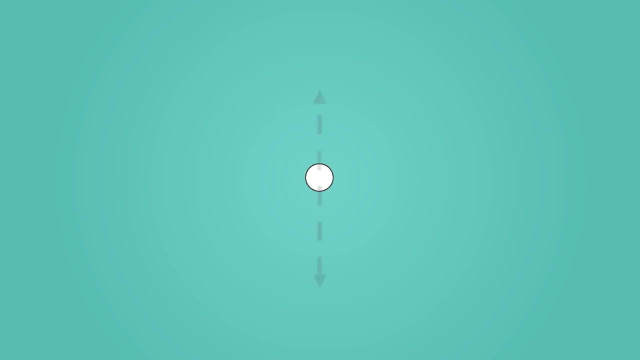 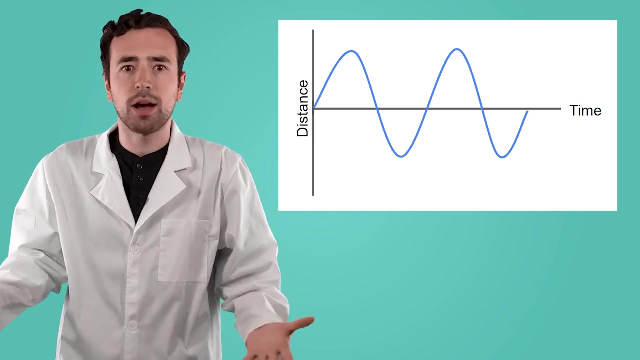 particle of matter. It begins at rest. then, when a force causes it to make a sound, it moves back and forth a certain distance. When we follow that movement over time, it's just a movement. We get this a sound wave. By looking at the shape of a sound wave, we can learn a lot about what a sound sounds like. 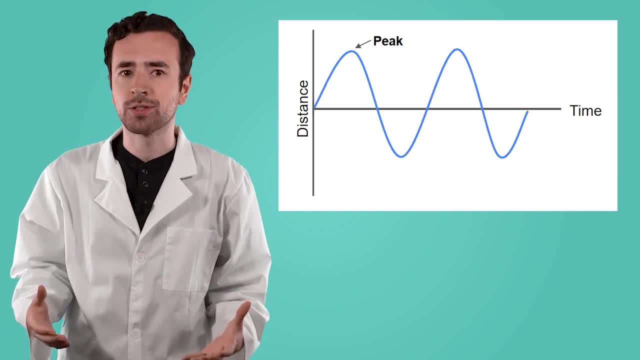 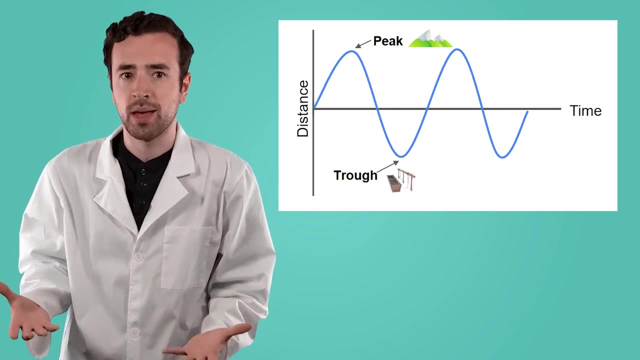 For instance, the top of the wave is called the peak, just like the top of a mountain, And the bottom of the wave is called the trough, like what farm animals drink from? How far a particle moves from its starting point to either a peak or a trough? 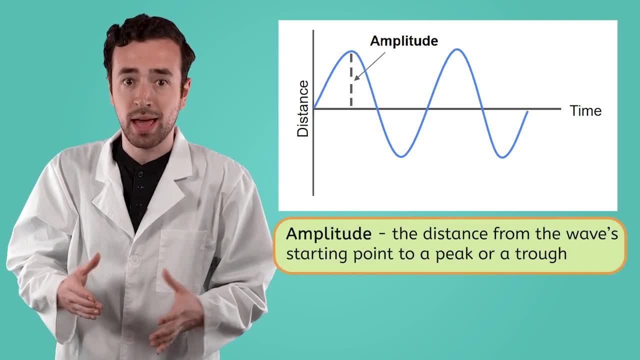 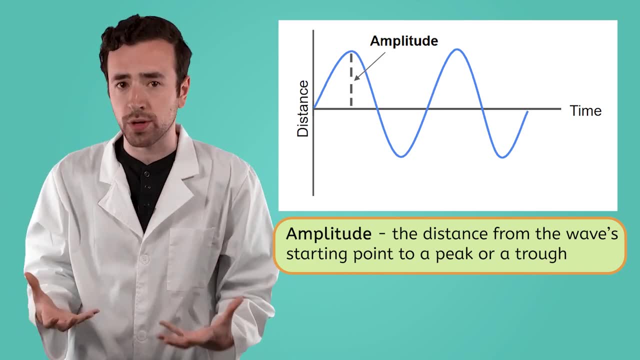 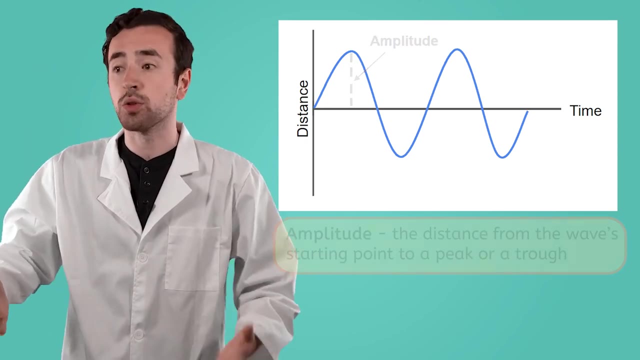 is called its amplitude. Amplitude shows us the strength of a sound wave, or how much energy was behind the force that created it. The more energy, the farther back and forth the matter will vibrate On a sound wave. more energy looks like taller peaks and deeper troughs. 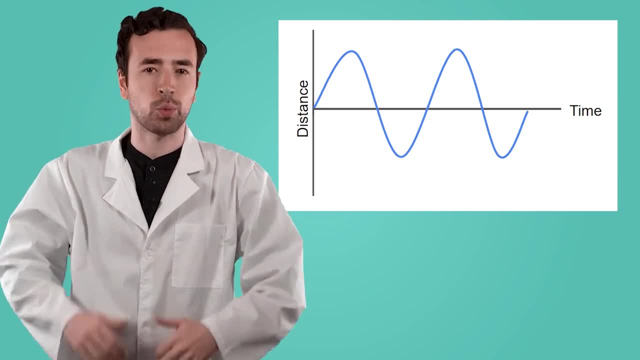 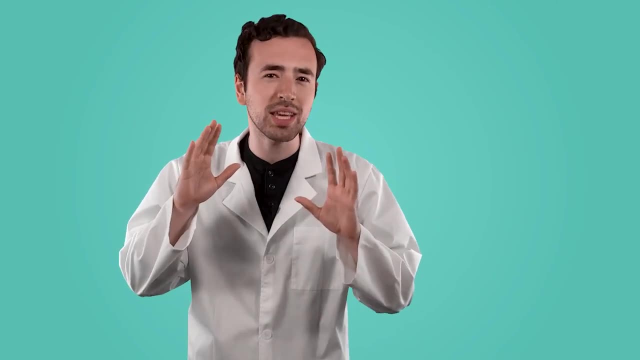 while less energy looks like shorter peaks and shallower troughs. How do you think the amount of energy put into making a sound changes the sound of a sound? How does it change how we perceive or hear it? Pause the video here and listen for the difference yourself. 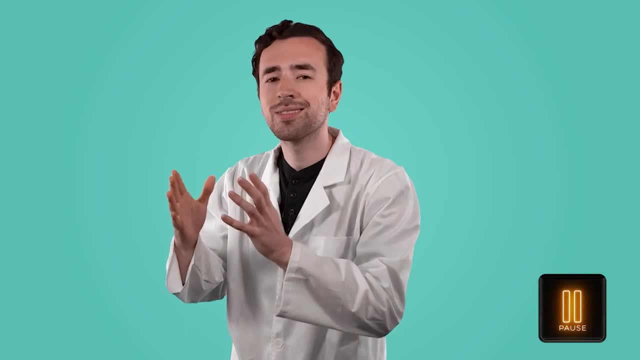 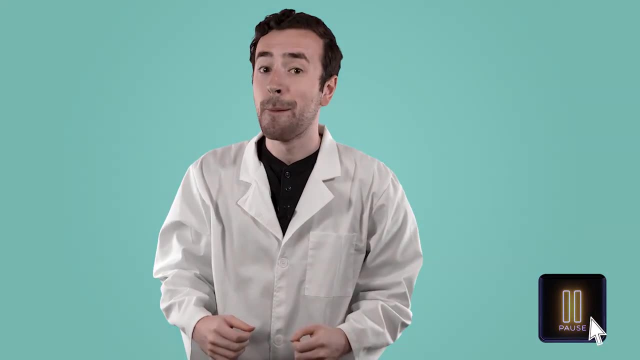 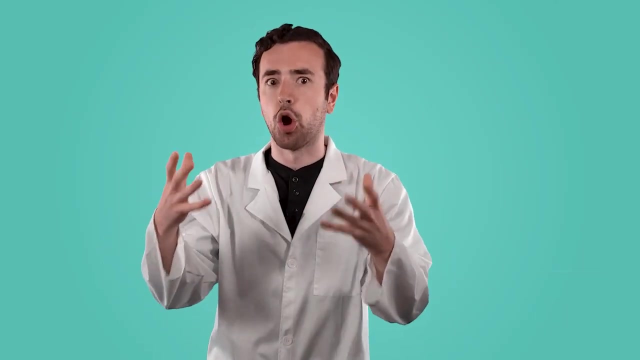 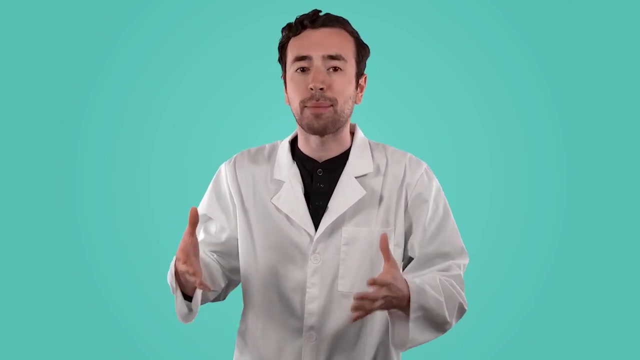 Clap your hands together once softly and once with a lot of force. Record the differences you observe in your guided notes. The sound of my voice currently has a large amplitude. Sorry, Sorry, Notice that when you clapped your hands together hard. 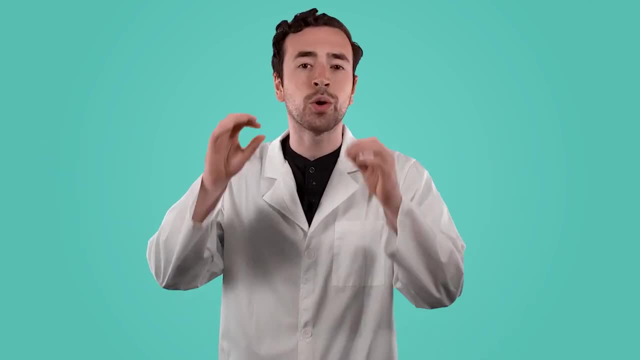 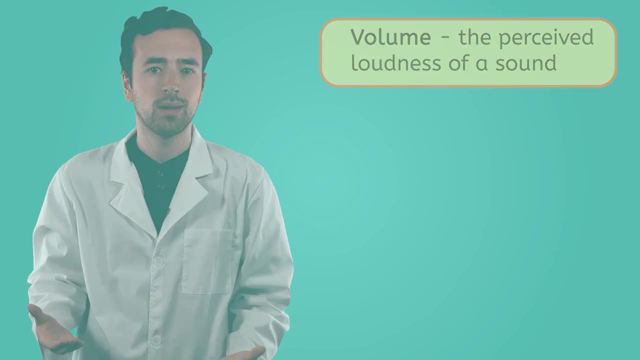 the sound was a lot louder than when you did it so softly. We perceive the energy of a sound as the sound's loudness or volume, So the amplitude of a wave tells us how loud or quiet the volume of the sound is. 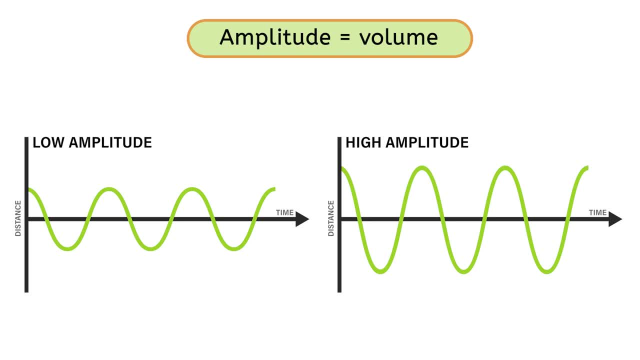 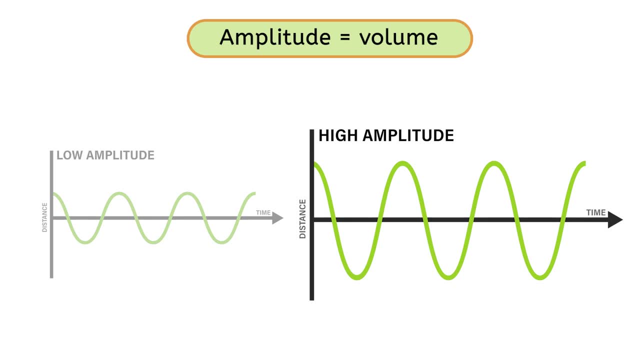 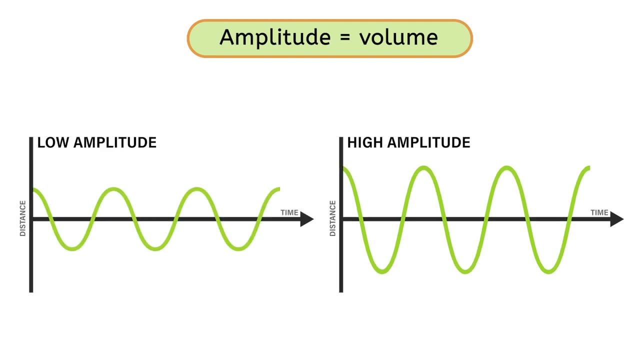 So which wave is showing a louder sound? Right, The matter is moving farther from its starting point in this wave, showing us that this is the louder sound. Which one is showing a quieter sound? Good, The wave with the smaller amplitude represents a quieter sound. 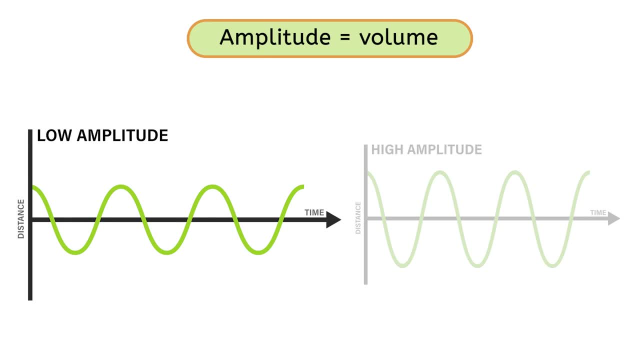 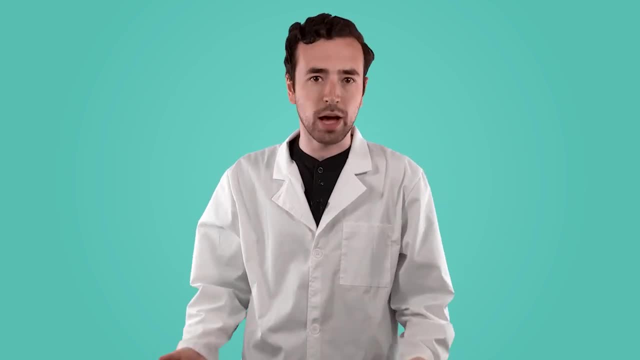 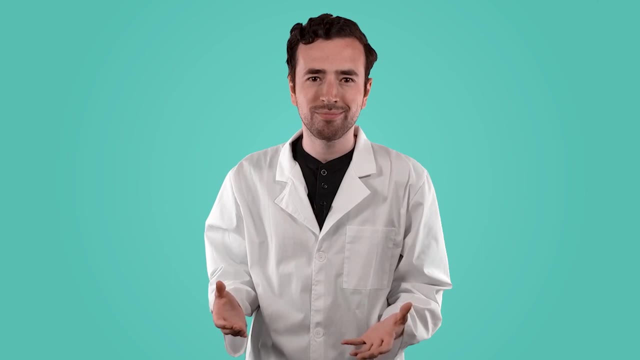 The amplitude of a sound wave shows the volume of a sound. Volume is not the only way we perceive differences in sound, though. Can you think of any other ways sounds can sound differently from each other? I don't know, But inедit. 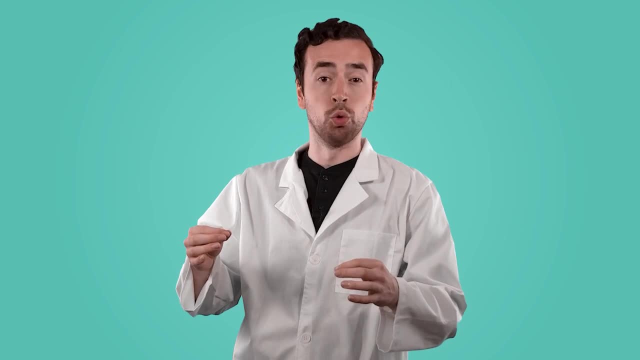 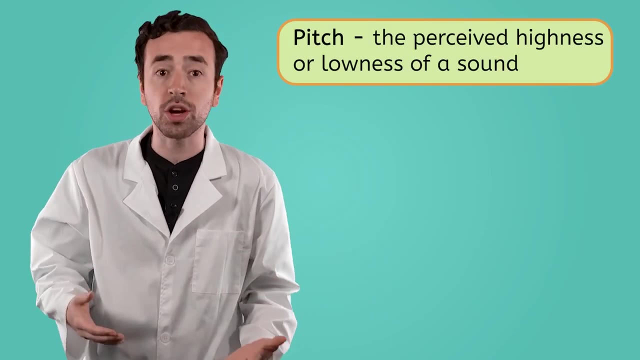 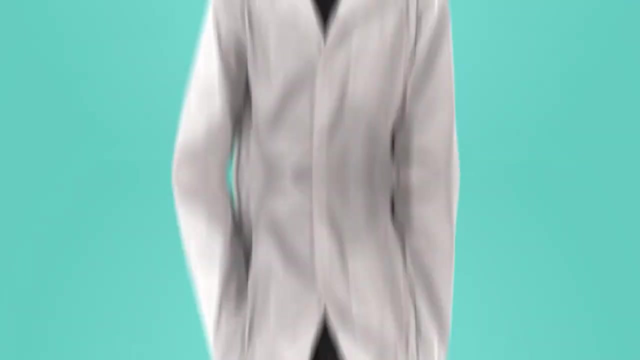 That's right. Sometimes a sound can sound low And sometimes a sound can sound high. The highness or lowness of a sound is called its pitch, and that's also something we can see when we look at a sound wave. 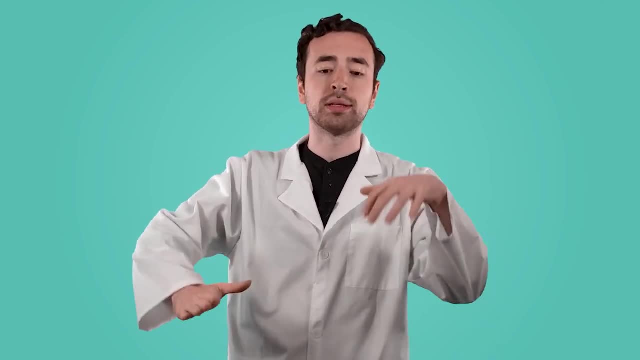 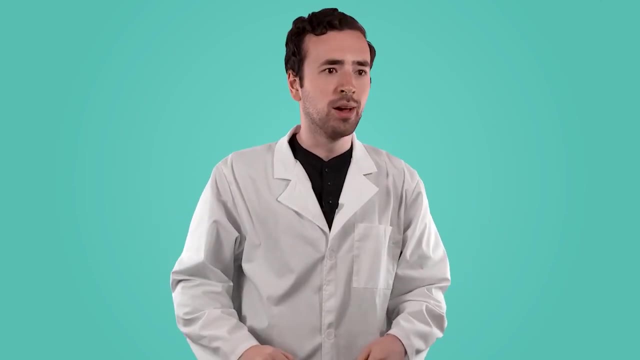 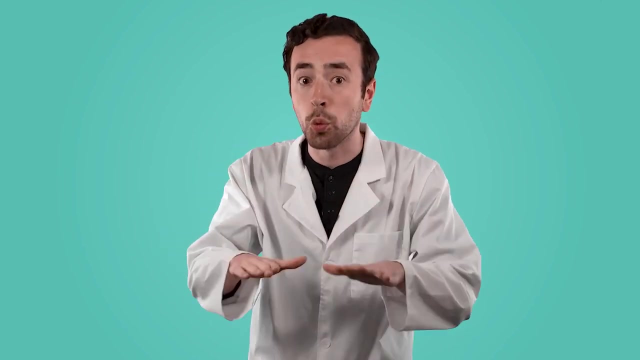 Have you ever noticed what happens to the sound on a video When you put it in slo-mo trying to watch a video quickly, so you put it on two times speed. Whoa, don't let me do that again. But did you notice how the pitch of my voice got lower when? 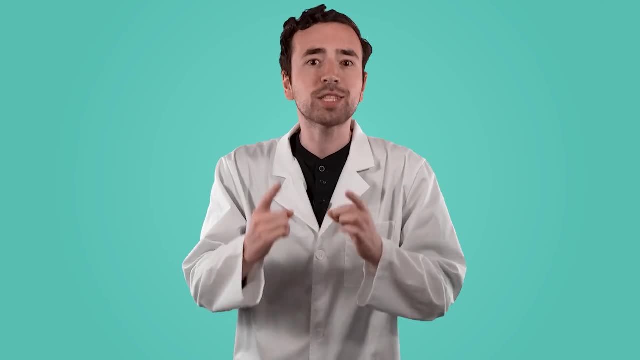 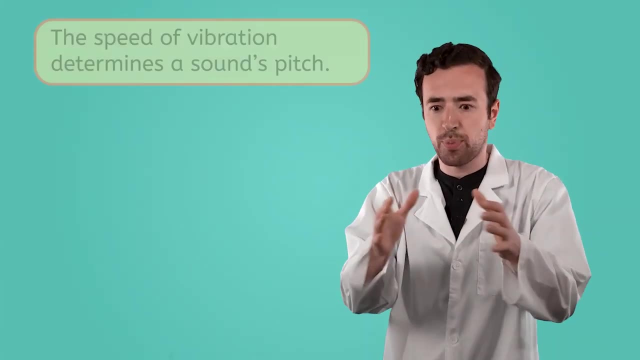 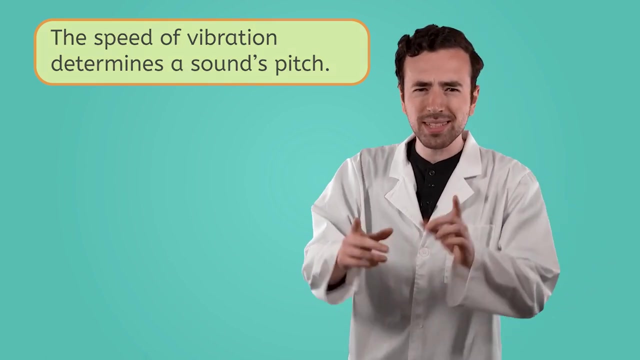 it was slowed down and higher when it was sped up. That's because the speed of the vibration is what determines a sound's pitch. When matter vibrates faster, it creates a higher pitch, and when it vibrates slower, it creates a lower pitch. Let's take a look at how we can see that. 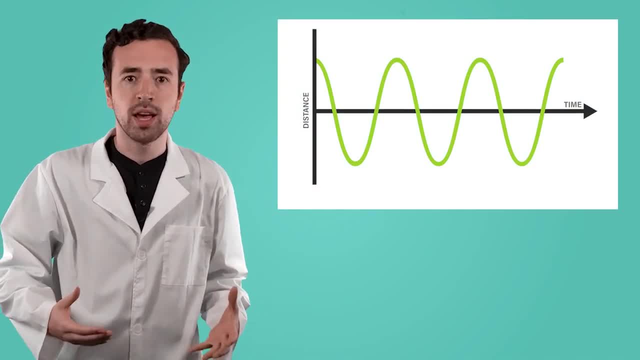 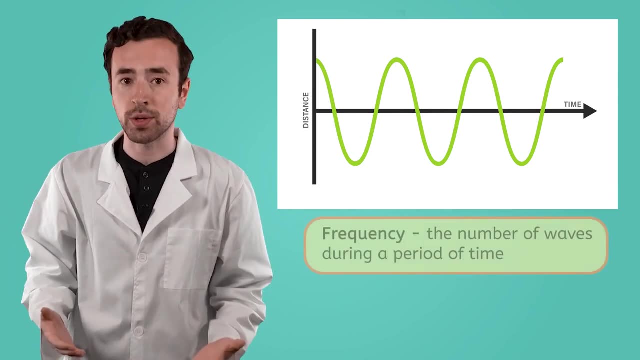 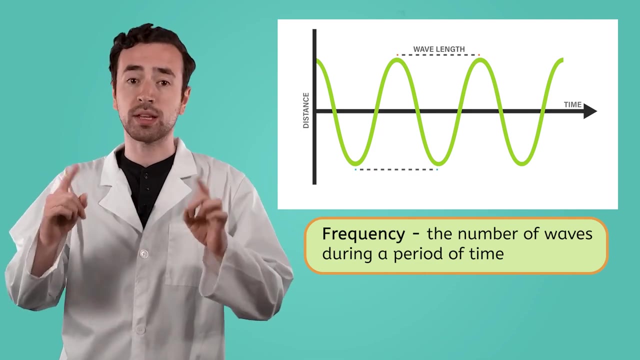 on a sound wave. The faster matter vibrates, the more sound waves there are during a given period of time. That measurement is called frequency. We could determine the frequency of a wave by looking at its wavelength or the distance between two peaks or two troughs A higher. 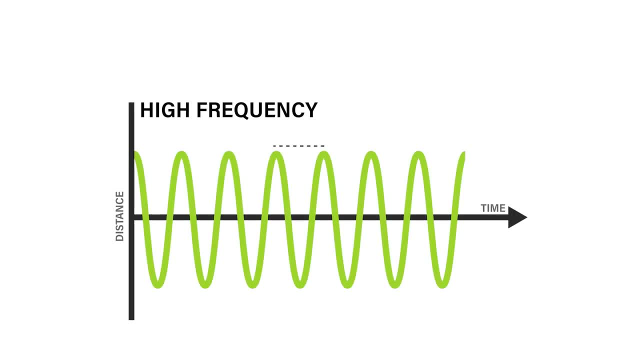 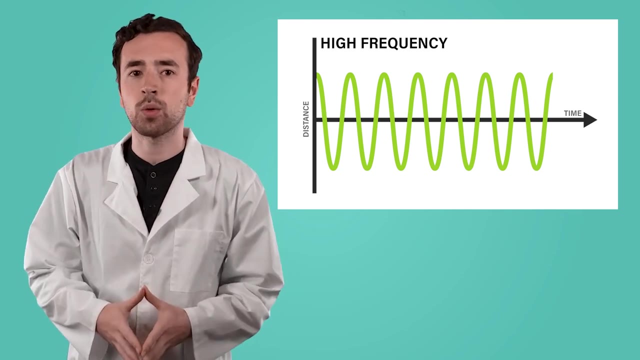 frequency means the wave has a shorter wavelength, which makes the wave look kind of squished together. A higher frequency creates a higher pitch. You can think of frequency like the word frequent. It's describing how frequently or how often something is happening. If a high frequency sound looks like a lot of waves close.